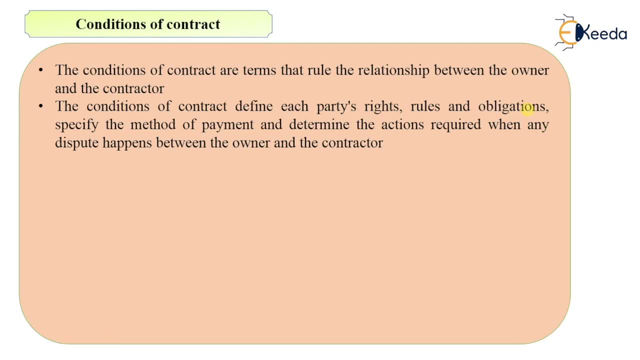 the completion of project, for the execution of project, for the supply of materials, supply of services, providing the services. All rules and regulations and obligations will be there. Then they will be mentioned in the conditions of contract. Then conditions of contract. 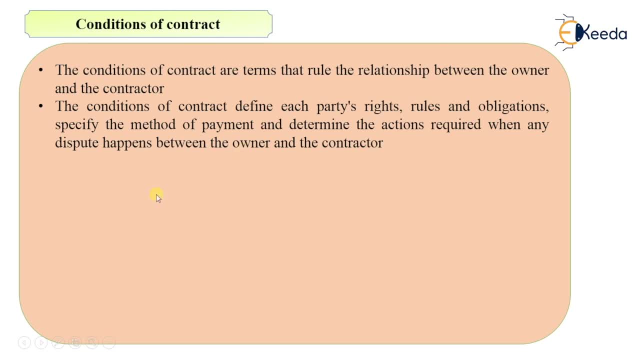 also specify the method of payment Means. in the conditions of contract there will be mentioned that the mode of payment to the contractor will be by cheque, by cash, by whatever it is, by any FTE, by bank, by any other means. So it will be mentioned what. 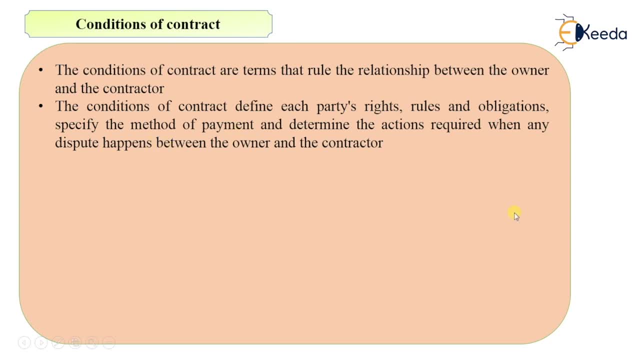 is the method of payment And as per what, What, How, How the particular contractor will be paid, Depending upon the work done: in meter cube for the brick works, for excavation, it is meter cube. for plaster, it is meter square. What will be the method of payment? That will also be included in the conditions of contract. 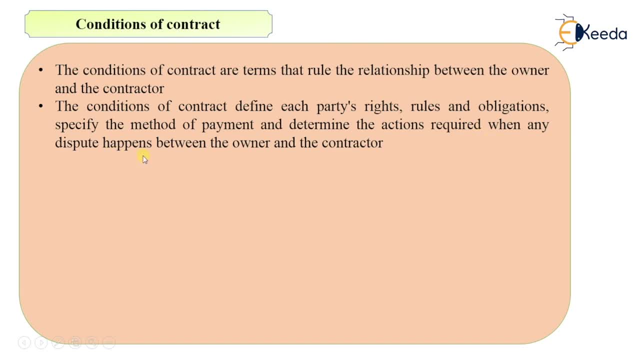 Then determine the actions required when a dispute happen between the owner and the contractor. It also determines what is the precaution or what is the action that you should take if any dispute happens between the contractor and the owner, So that are mentioned in the conditions of contract. 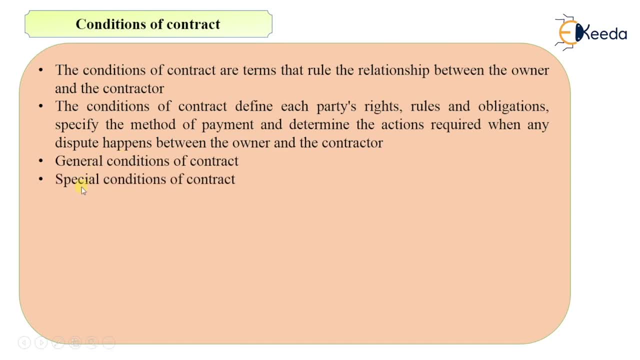 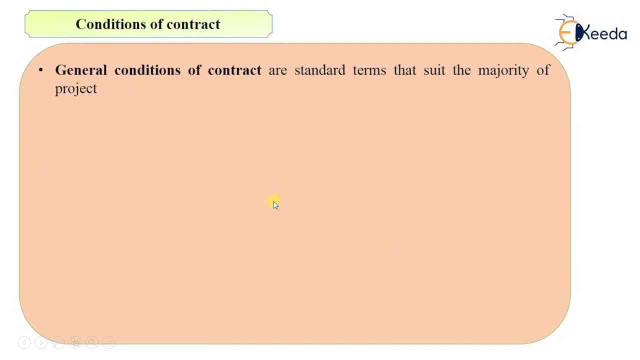 So we have general conditions of contract and we have special conditions of contract. Let's see them one by one. First we will see the general conditions of contract See. general conditions of contract are standard terms that suit the majority of project. They 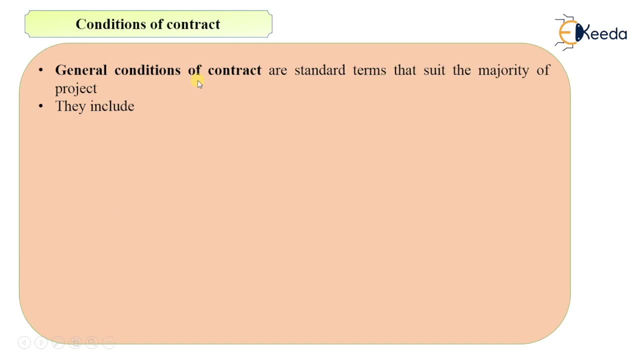 are general contracts And they will suit majority of the projects, Means they will be similar for majority of the projects, such as definition of project contract components, then rights and responsibilities for the owner and the contractor. They are general means. you can say copy paste material. 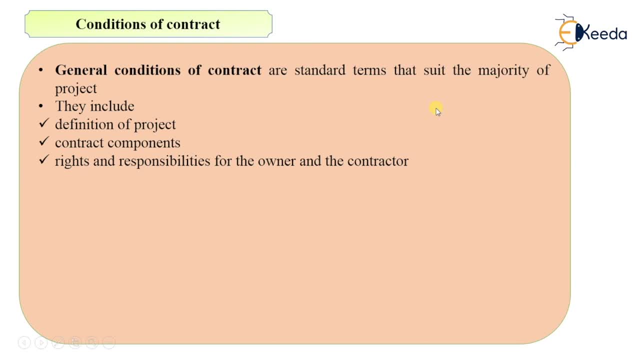 they are. They will be applicable to majority of the project. so many projects, Then project schedule. payment method, then delay penalty. so these are included in the general conditions. what are include what? what they will include? they will have definition of the contract or project. what is the type of project? how big is it? 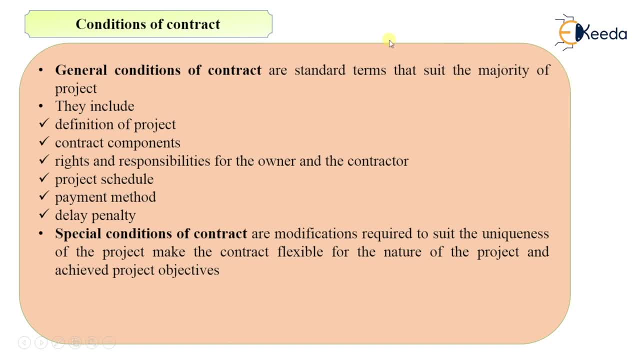 what is the type of project, whether it is a construction of a public building, residential building, whether it is a construction of dam, reservoir, culvert, minor bridges, major bridges, whatever it is. so it will define the project, what exactly the project is and their conditions, in which situations they it should be completed, in how much time it should be completed, what if. 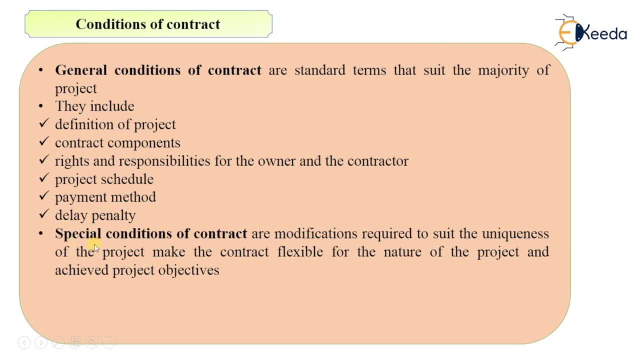 the contractor delays the work, there will be delay penalty. that will be mentioned in the general conditions of contract. payment method, as i told you in the previous slide. then project schedule: in how many, how many months, how many years, the complete project should be completed. that project should be completed. that is mentioned in the general conditions of contract. 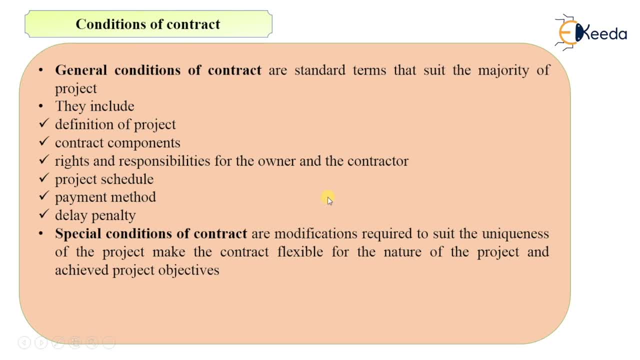 what are the rights of owner? what are the rights of contractor? what are the responsibilities of the contractor at the time of execution the work? so all these are mentioned in the general conditions of contract. then we have special conditions of contract. see, these are the modifications required to suit. 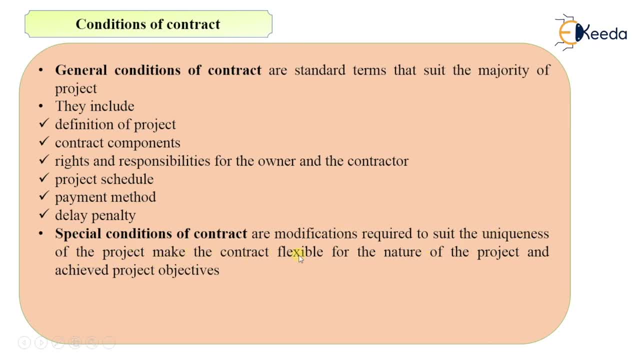 the uniqueness of the project, make the contract flexible for the nature of the project and achieve the project objectives. there are some conditions which are not applicable to a certain specific project. so these are the conditions of contract. see, these are the modifications required to a specific project, so we have to modify them and make them special conditions. 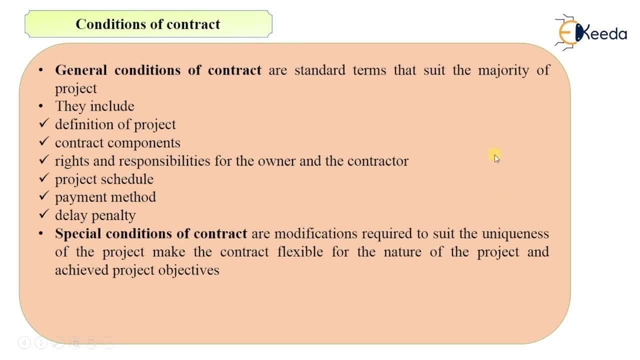 so those conditions will be known as special conditions, means that conditions, the general conditions, which are modified as per the requirement of a project- it is not a general project, is maybe it is a special type of project- that general conditions will not be applicable at this, at that place. so we will have to use or we will have to modify the general conditions. 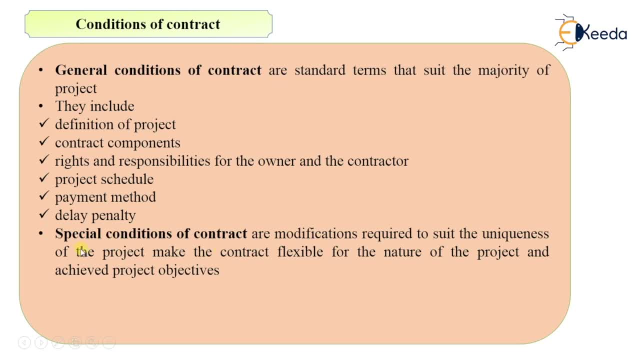 to make it special conditions and those. those conditions will be called as special conditions of contract and they will suit the proper project objectives. what will be the objectives? what are the objectives of project? depending upon them, we will modify them as per our requirement. then special conditions.